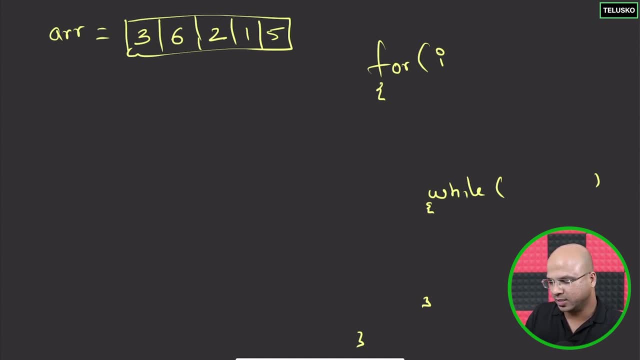 going to create a variable. we are going to use one variable, but let's also go for J. So we need a I variable. let me just write I here. we need a J variable and we need a key as well so that you can store this value somewhere. So at one point you will compare and you will save it. Now, from where we are going to start this Now, if you want to understand what what we're going to do is where? it's very simple. So initially you will take your six as a key. So when you write this variable, we'll say key is initially six. 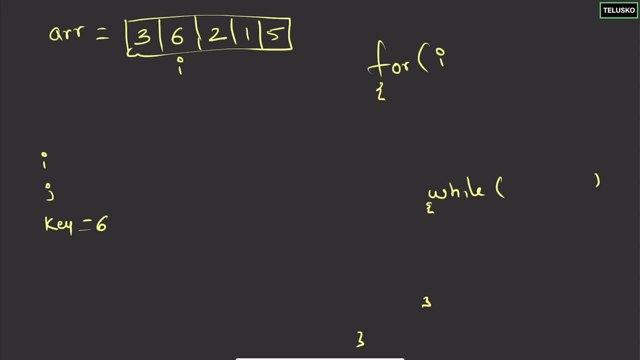 Okay now how you're going to get six. So let's say we take a variable I here, and then we'll keep the J here. Okay, so we're not going to start I from the first one, we're going to start I from the second one And then J will be the first value. Now I will represent the outer loop and J will change in the inner loop as well. Okay, so that's why we are going for I and J. we could have gone for different variable name, but we got used to I and J for the outer loop and inner loop. Okay, so now what you're going to do. So the idea is very simple. Once you've got 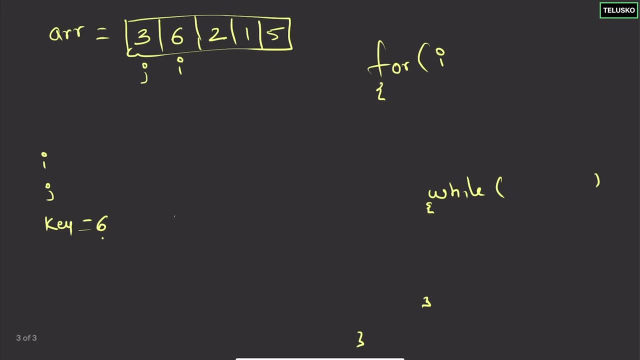 a key which is six in this case. now how you got six? maybe we can do something like this: we'll say ARR of I, whatever I represents, we'll save that in the variable key, And then we're going to start J by saying J is equal to I minus one. So I is starting from one, So J is I minus one. That means the value for J initially will be zero And I is one. Now, what you're going to do with this? it's very simple. you will simply compare the value of J, which is this the 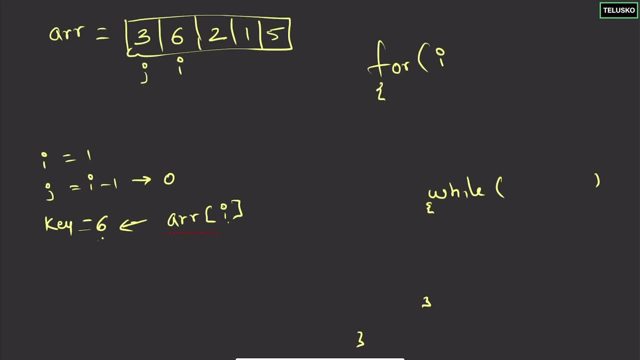 first value. So we'll compare J with the key. If this value is greater than the key, then you will do the shifting part. At this point we don't need that right, Because the value of J, where the J represents, is less than the key, then you don't have to do any shifting part. So this is already sorted, Okay, But let's go for the next iteration. Now, when you're sending next iteration, it's very simple. What you simply do is so you shift your value of I here and you shift your value of J here, because we know that the three and six, if you compare this to: 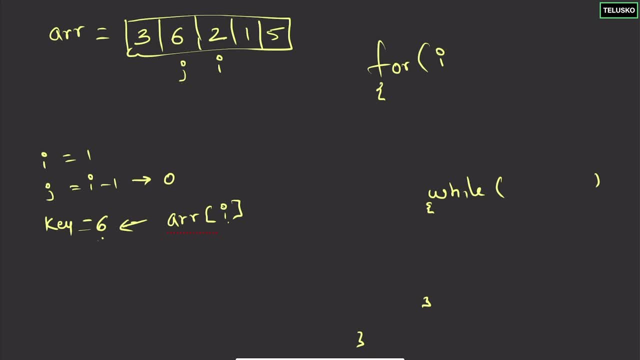 they are sorted. Let's go for the next one. Now, in this, what you will do is you will check again, you will change certain things, right, If you can see. this will change, because now ARR of I is not six, ARR of I is basically two. Okay, so key is two. now What about the value of I? even I is changed. I is now two, So index is two. So let me also write index so that it will make much more sense. right, So that those are the index value. So I value is two. now What about J? So J is I minus one, So J will. 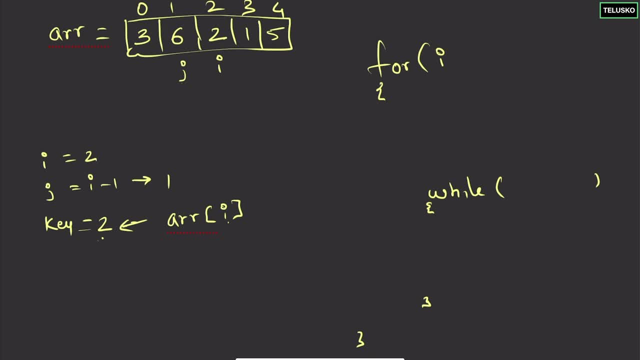 start from one. So J is I minus one, So I will start from one. So J is I minus one, So J will start from one. So J is I minus one. So J will start from start from 1. that's done, and now you will apply a condition. so what, basically, condition we are? 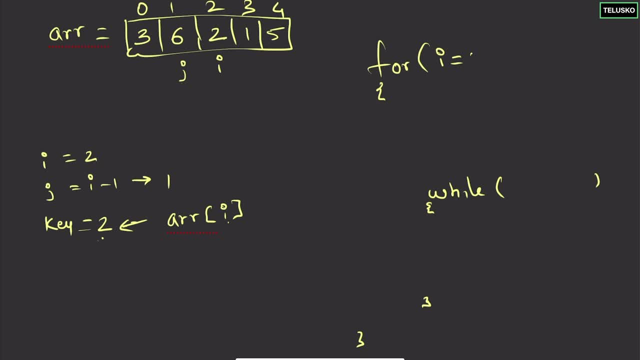 checking for. so, of course, if you write the code here, so i is initially starting with 1, we are now starting with 0, and then we'll go till i less than n, if the value, if the length of this array is n, and then we'll say i plus plus, okay, and then we'll assign the value. okay, we'll, let's not write. 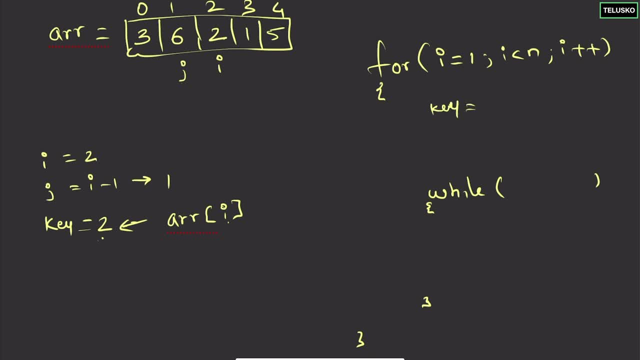 the actual code. let's write some dummy code. so let's say we got a key variable. the value for key is basically arr, which is the array of i, and that's what we are doing here. that's one thing. next, we also need j variable. so we'll say j is equal to i minus 1. okay, that's how we're going. 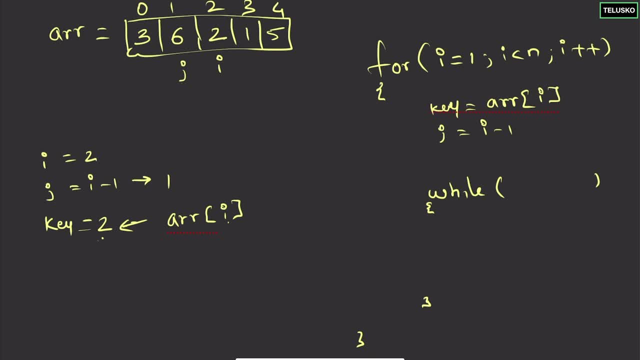 to start now, what you're going to compare in the while loop. so in the while loop it's very simple. you will check for the arr, so arr of j, let me just say i'll complete this here. so this: if this is greater than the key, because the shifting part will come only when 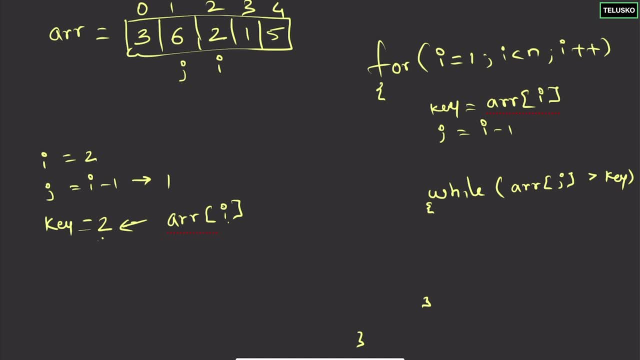 whatever is represented by j is greater than the key. so, if you can see, the key is 2 here and in this case, yes, it is greater, so 6 is greater than 2. so what you do is you basically perform some operation. now what option i'm going to perform? so basically, first of all, i will take: 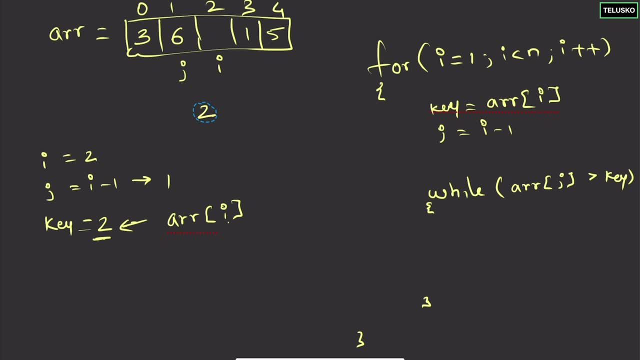 this key somewhere. of course we are storing that key 2 in the key variable, and then you do the shifting. shifting of what? so you will first compare this 2 with 6, and now we know that we have to shift 6, so you will shift 6 here. then that's one done, right. 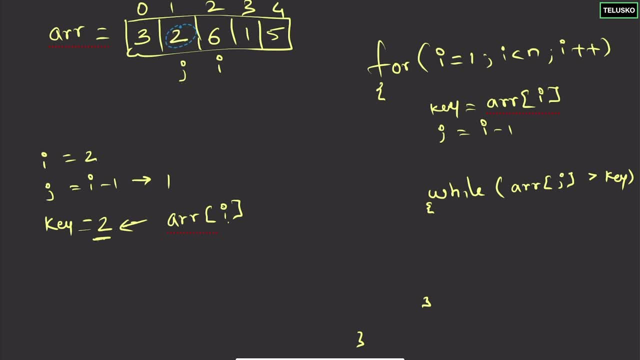 can you put 2 here? we can, actually we can put 2 here, but the problem is, we also know that we have to compare 2 with the previous value, which is 3 in this case. so you will not shift 2 there, but we'll shift 3 here. but then to shift 3 here, what we have to also do is we have to first shift. 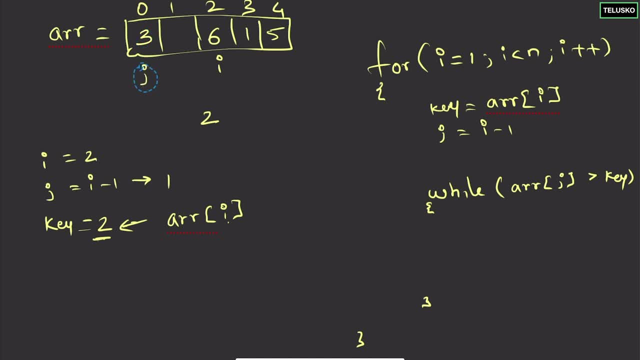 our j here on the first location. that means we are also going to perform j minus minus, right? so what i'm saying is, the first option you're going to perform is shifting the values, right? so how do you shift? you simply take the next value. so initially, j was. 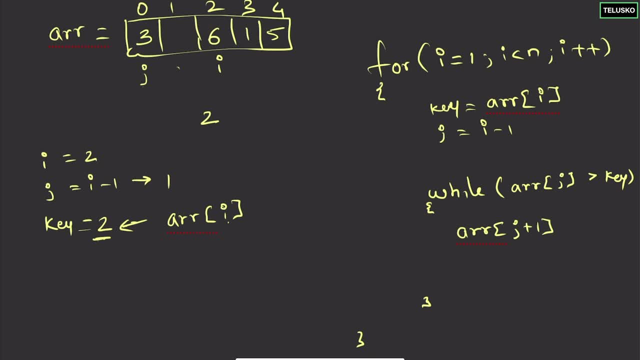 here, right? so this value 6 is going here. so that means what we can do is we can say: arr of j plus 1, which is in this case 2, is arr of j. by doing this, what you're doing is you're shifting so the 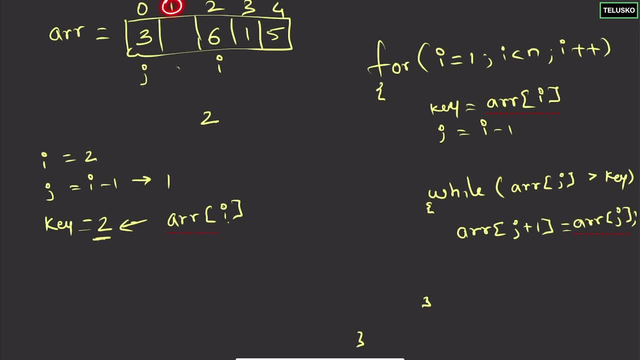 j initially was here, which is 1, so index of j was 1, or the value of j was 1. then you're saying j of 2, i mean j becomes 2. then what we are saying is we are saying j plus 1, which is 2, so the value of 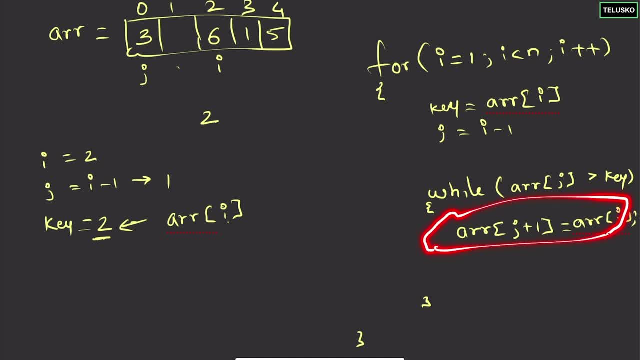 6, which was here, will move here. that's what we are doing on this line. so this is the entire logic. you have right, but this loop will repeat right now, when it will repeat. look at the condition here. the condition is whatever j, so we are shifting j backwards, right? 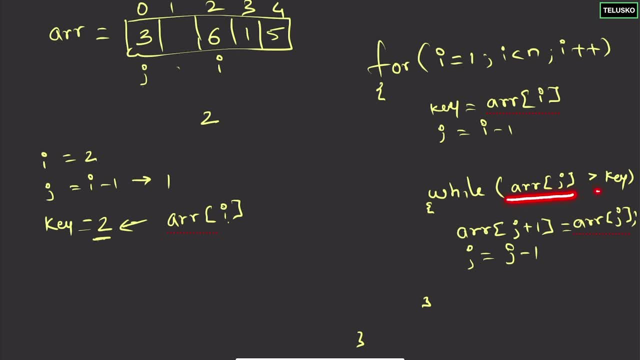 j is now here, so we'll check if arr of j is greater than key in this case. yes, you can see the key is 2, arr of j is 3, so it is greater. so we'll shift. so how do you shift? basically, you do the same operation, which is the inside of the loop, so you can see that you have a loop. 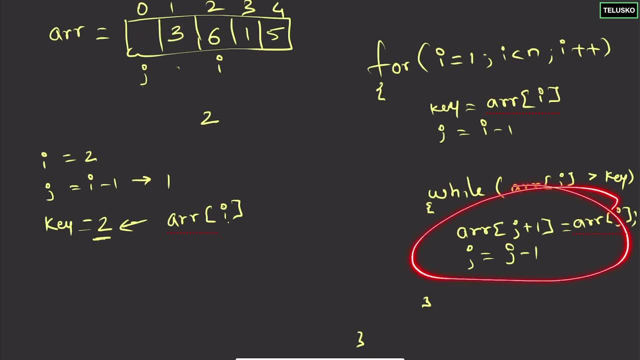 inside the while loop. so if you compare this operation, this is what it is doing, the shifting part right. and then we know that, of course, if you can see, here we have one more step. you will do j minus 1, which means your j basically moves 1 here, because when you reduce the value of j it becomes 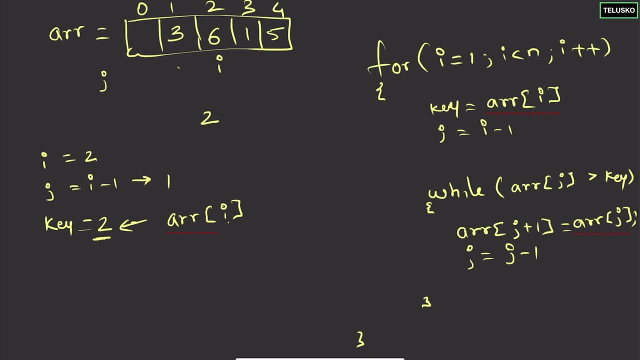 it became 0, right, and then again you're doing it. so it will become j. j becomes minus 1, so we have to stop it here. once the j becomes less than 0, we have to stop. but don't you think we have to also add that condition in the while loop? so we'll do that, we'll. 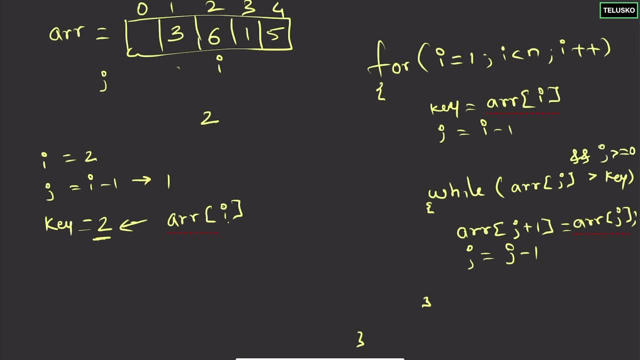 say: and j should be greater than equal to 0. okay, this is one condition we have to add. if this is false, if j is not less than or equal to 0, then you will do the last, last step. the last step is very simple: you move your 2 here, and the way you can do that is by saying arr of j plus 1, because 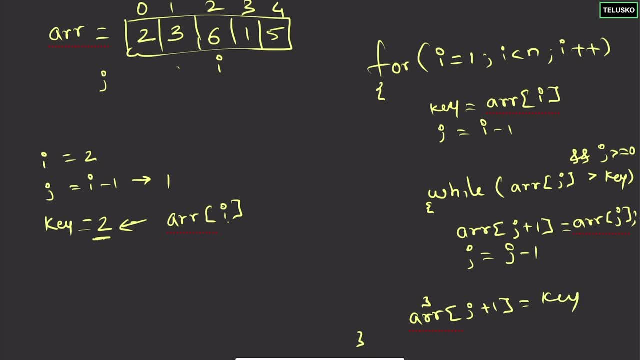 j became minus 1. we don't want minus 1, we want 0 is equal to k is equal to key. so, basically, this is where the value goes first. now, by doing this, we were able to sort the first three values. now what next? of course, you will increment the value of i. 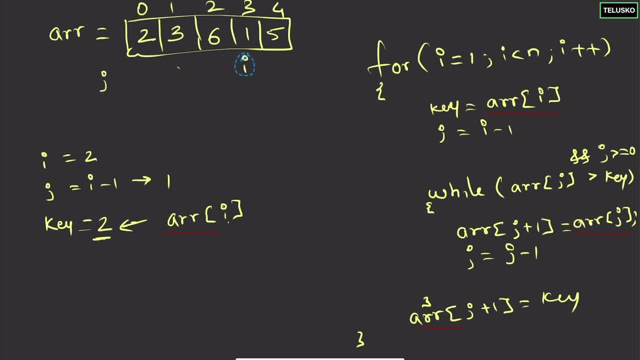 you say increment, that means the value of the i variable goes here and again. for the next situation, j goes, i minus 1, right because of this? basically, for the outer loop, the i value is incrementing but the j value is just before i. and again you, just you do the same things. what are the? 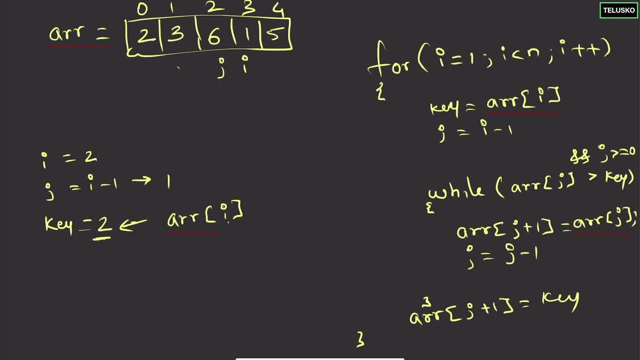 same things. you first check if the key. okay, we have to update the key as well. now, how do you update the key? now? the key value is arr of i, which is, in this case, should be 1. so the new key is 1, i is 3 and j is 2. okay, new key value is 1. you will compare if the arr of j. this is the condition. 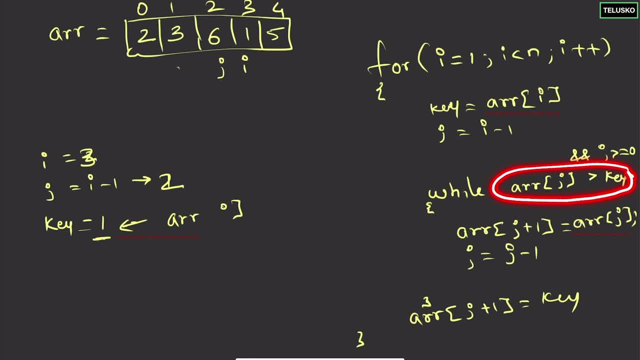 we're checking now if arr of j, which is, in this case, is 6, is greater than the key in this case. yes, you perform this operation. what is the operation? it's very simple. let's keep this value somewhere. you start shifting 6 here, 6 goes there, and then your j comes back. j comes here. 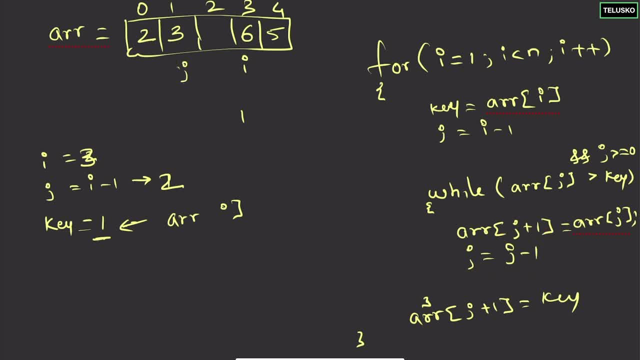 right because of this step here, right. and then you, you again check if arr of j is greater than key. yes, 3 is greater than 1. again, you will shift 3 here, then you shift j here, then again you shift 2 here, then you shift j here, and then now j becomes. 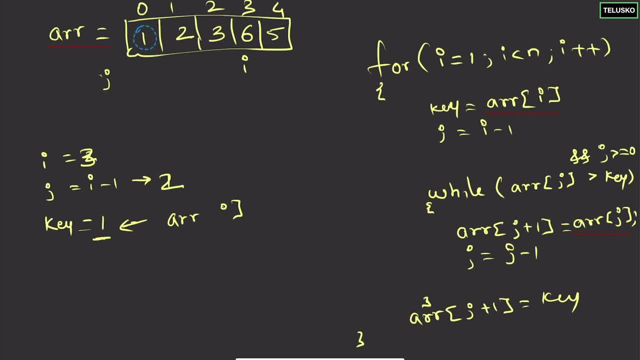 minus 1. let's stop the loop and shift 1 here. you can just do the same thing for 5. let's do that quickly. so what you will do is you will shift the value of i here, which means certain things are going to change now. this i becomes 4, this j becomes 3. the key value now is 5. 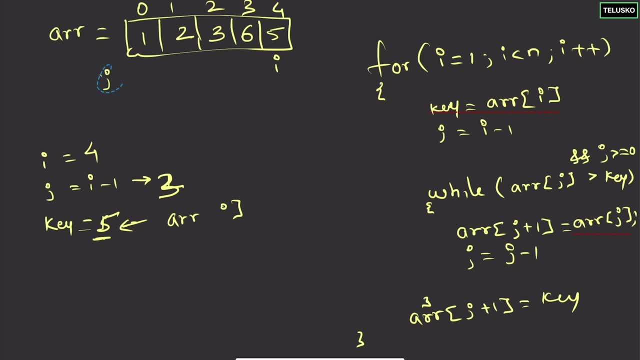 right again, you do the same things. you keep your j here, because j is just i minus 1. then you compare if the arr of j, which is 6 in this case, is greater than the key. yes, let's do the shifting. now, how do we do that? let's move that here. and then we have to shift 6 here. j goes here. now again you check. 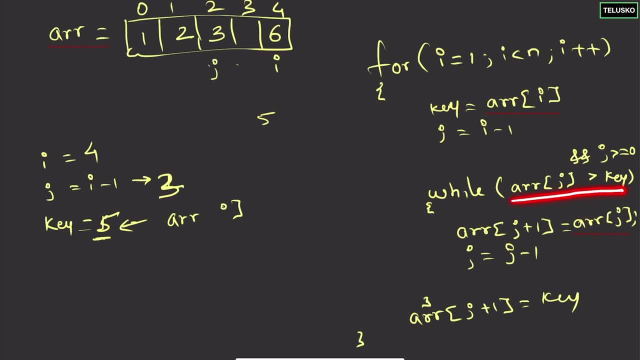 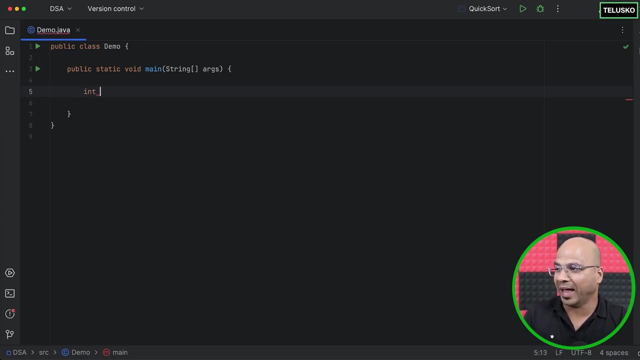 is the arr of j is greater than key. no, it's not there, so you will just simply come out of the loop here and, if you can see, it's all sorted. so this is the logic. let's implement this logic in the code now. so let's write the logic. it's very simple. you create a array, so let's say this: 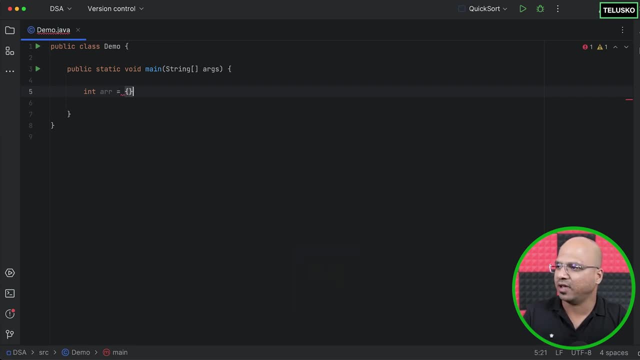 array is, arr is equal to. let's have some default values to it. let's say 5, 6, 2, 3, 1. this time we are going for only 5 values and this is an array. okay, what next now? basically, as we have written in the 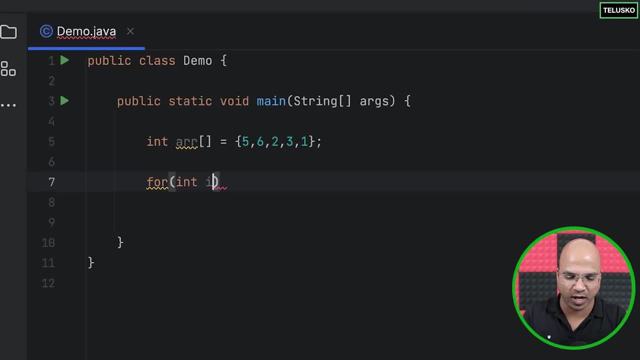 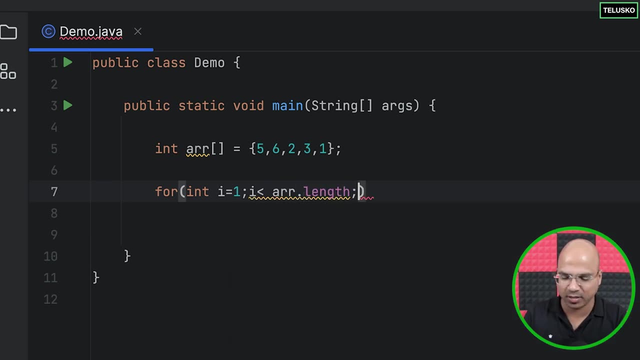 board. let's take a for loop now. the for loop is going to start with i. i is equal to 1 and we can now it will finish at n, but we don't know what n is. so we can say added dot length and we can say: 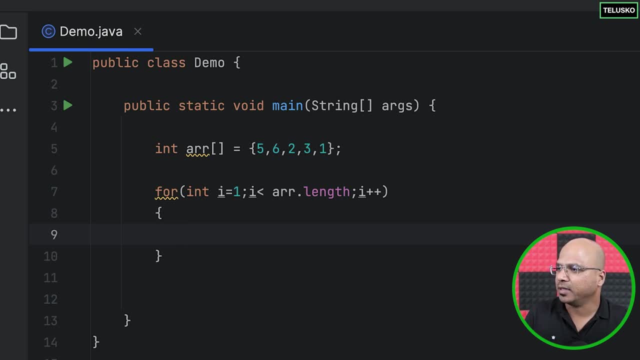 i plus plus. right, that's one done. and now, okay, let me just remove some space in between. okay, now, what are the extra variables we need? basically, we need two variables, right, we need key. the value for key will be arr of i, which we have done earlier. and then we also need j, and we know j is. 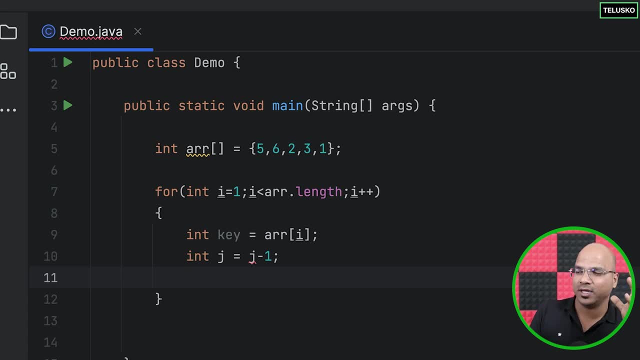 j minus 1. you know this. this is what happens when you know the algorithm on the on the board. right, i have a, i have a board with me, so, okay, those are the things we need. okay, not j minus 1, it should be i minus 1. and then you do a while loop, because this is where you do the iteration we have to. 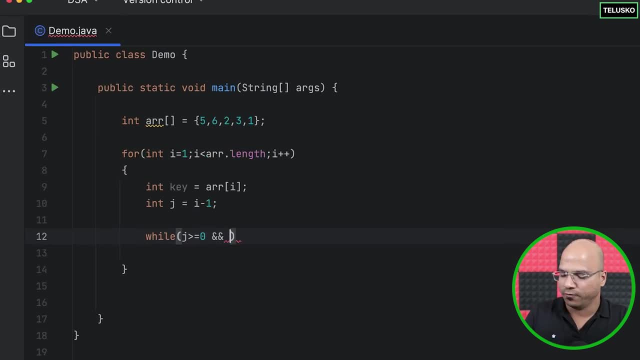 make sure that j is greater than 0. that's one thing. and we need to also check if arr of j is greater than key. in that case, you will execute the while loop. so you will do certain things here now what you are going to do inside this while loop. so, basically, you have to do the shifting.